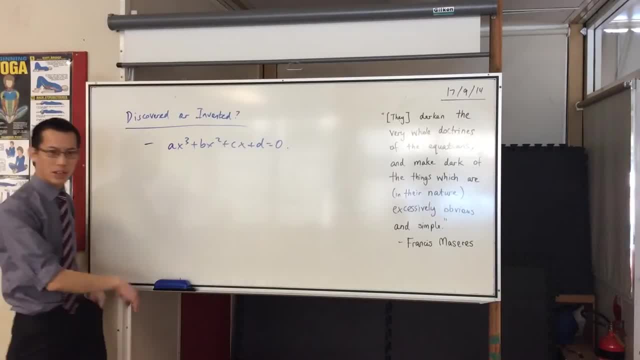 they're not hard to understand. Like we've looked at cubic equations before, I could give you something that would expand out to a cubic equation, But cubic equations are actually very difficult to understand. The maths of cubic equations is super hard. Right, If I gave you this. 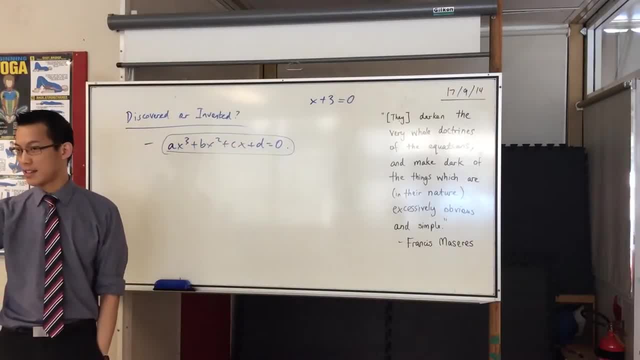 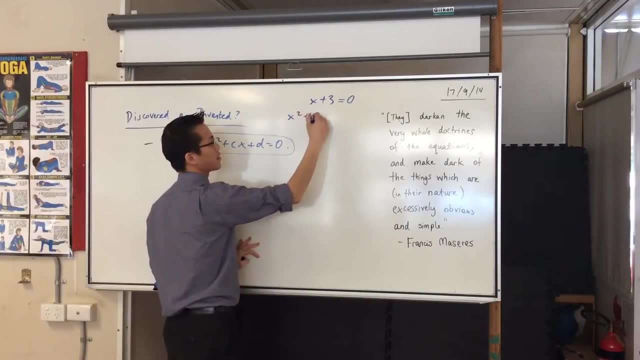 This is a linear equation and it's super easy to solve. The solution is: x equals negative, 3. Right, No problem. Like you, don't even need to do any work here. In the same way, something like this would take a little more mental effort. 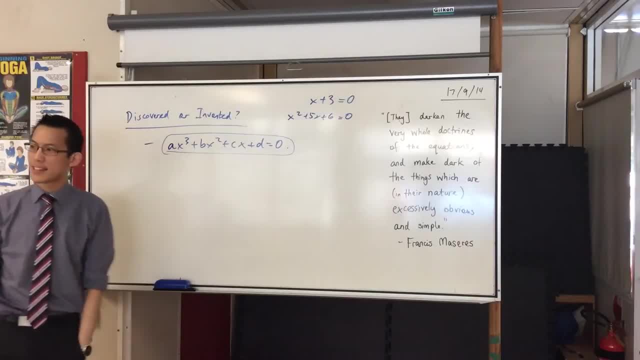 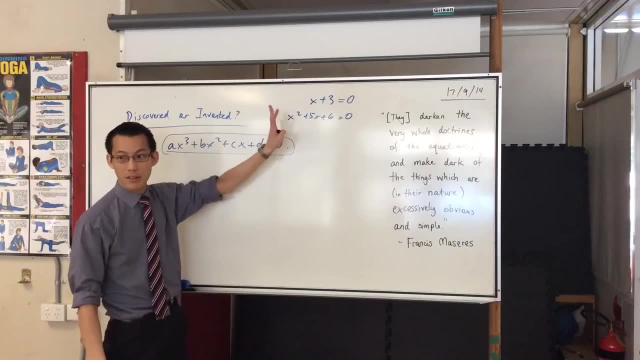 right, But you can solve this. Quadratic equations: we have well established the ways to work with these things, right, And so had ancient mathematicians like the Greeks and all that kind of thing. They understood all of this. That was fine. 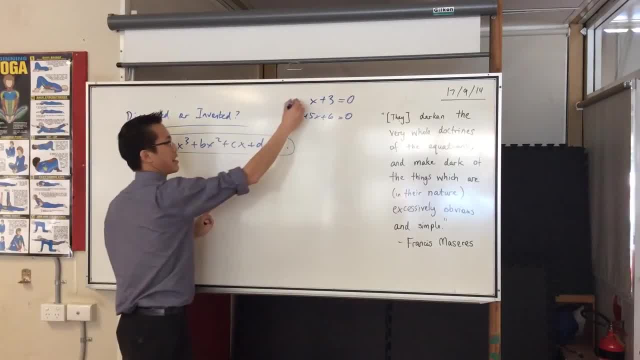 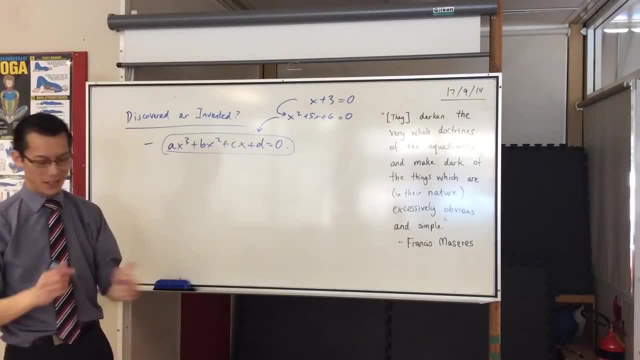 But you just step up one more time- Step one, step two- and everything explodes. People were working on this for centuries, And what was really cool is this is I don't know if they should go back to this kind of idea. 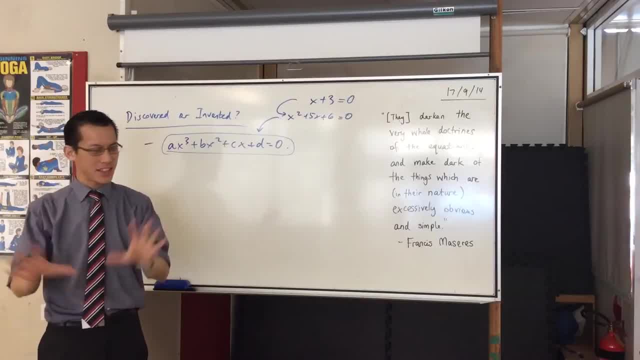 but in the past, particularly like in the Renaissance era, if you were like a teacher or a professor or something like that, the way that you got a job was you didn't apply and then have an interview- The way that you got a job, if suppose. 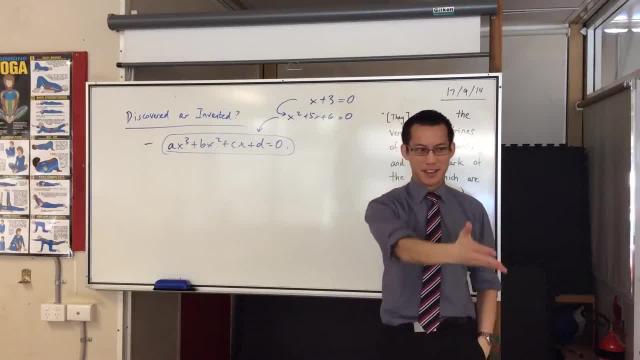 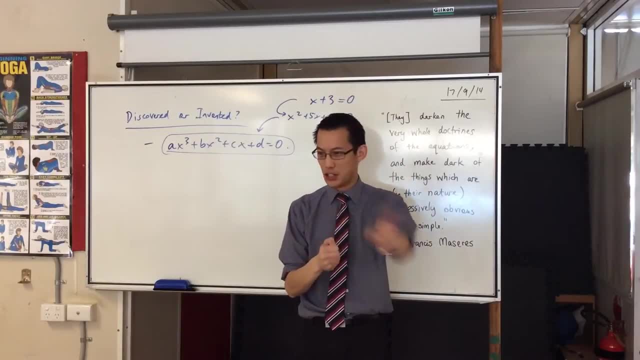 Jack was the current headteacher of maths or something like that, and I wanted to take his job. the way that I would do it is: I would challenge Jack to a duel right, I would write some questions. it would be a maths. 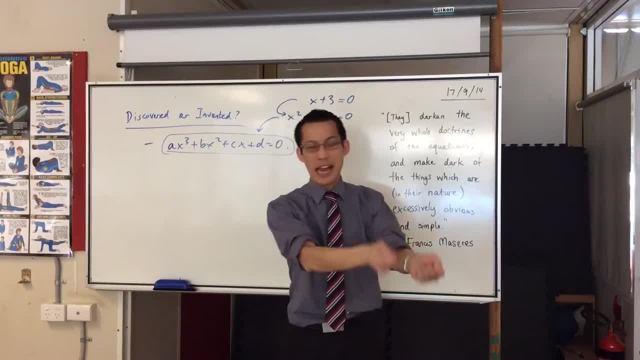 duel right. I'd write some questions that I know how to solve and I'd give them to Jack and Jack would do the same right And we would see who would win. So it was kind of like the more you know. 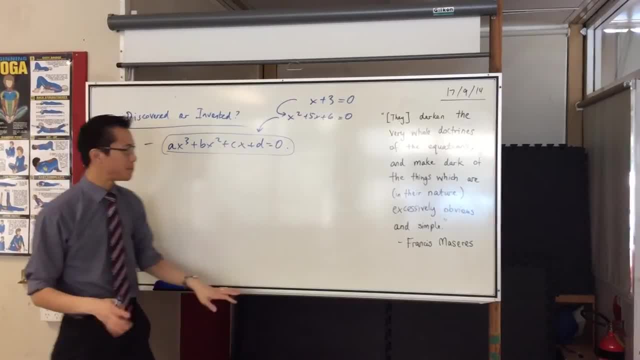 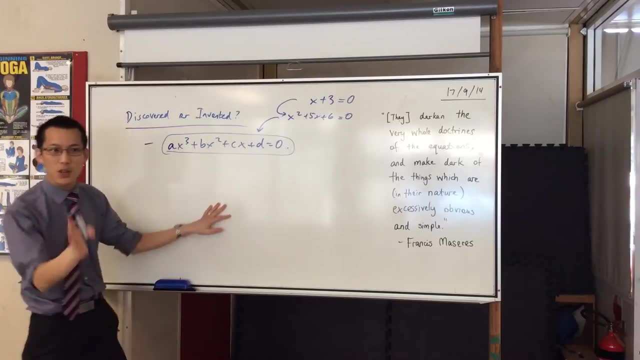 that's how you fight it out, and whoever can answer more questions is the winner. right Now, these kinds of questions appeared in these duels, these kind of tournaments, these matches, right, And it was kind of to your advantage, a bit like in a real 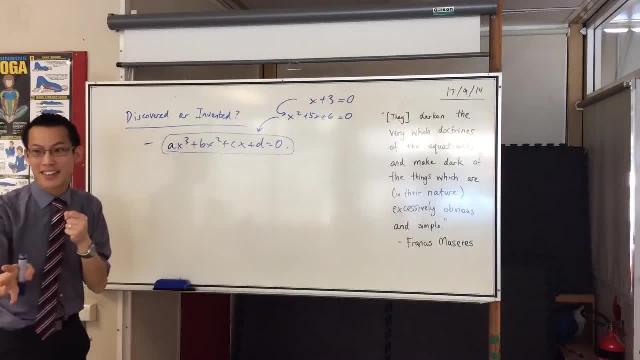 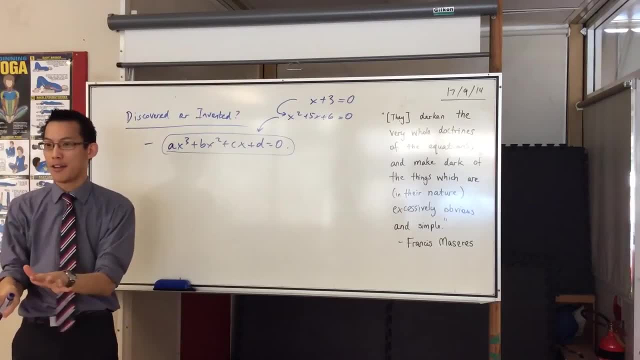 fight. if you know secret fighting techniques, right, that the other guy doesn't know, it's like I know this weird nerve pinch that I can do that will paralyze you or something, then you keep it to yourself. right, You find them out. 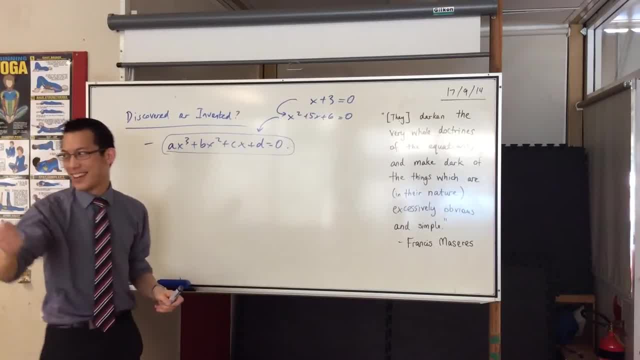 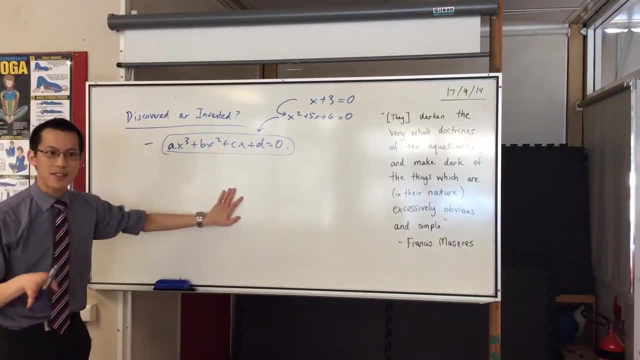 and then you're like I'm going to keep this in my back pocket and I can whip it out when I need to and I can fend off any challenges, right? So the ways to solve these kinds of things they were viewed kind of like and this: 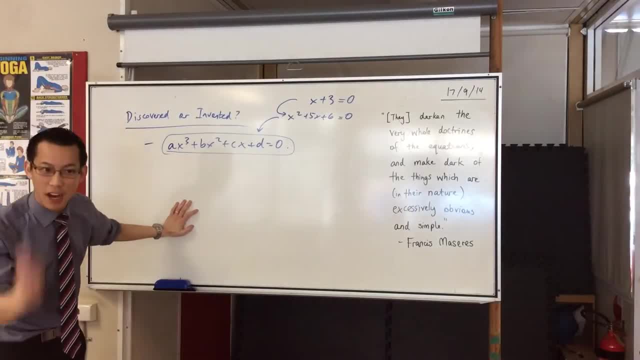 is the word that the presenter used when we were talking about this. they were kind of like discoveries that you could make about different kinds of versions of these you could solve and how to solve them right, And it was a bit like I said, it's like an arms race for who could solve them. 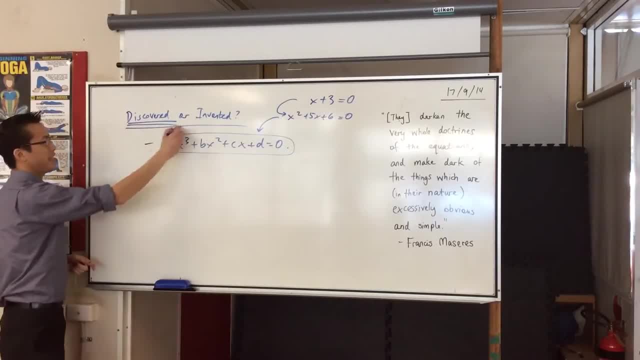 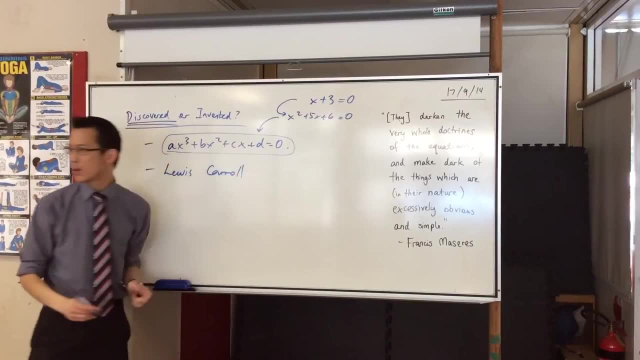 faster. So when you look at it from this point of view, it's a discovery thing. okay, Now there was another session I went to and he was talking a lot about Lewis Carroll. you remember this? Why were we looking at Lewis Carroll in the last few weeks? 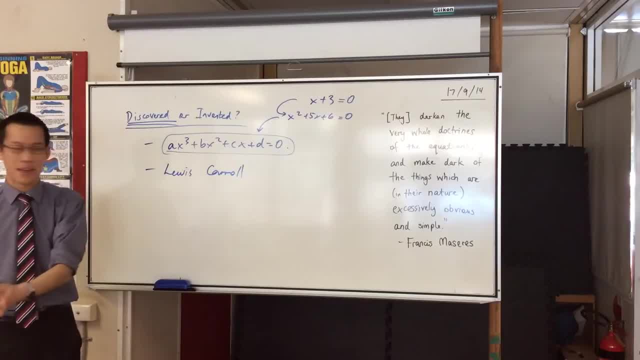 Carroll diagrams, which are an alternative to Venn diagrams. you remember that right. So he didn't just write Alice in Wonderland, he did a lot of maths, okay, And one of the interesting things that I attended that I got in this session. 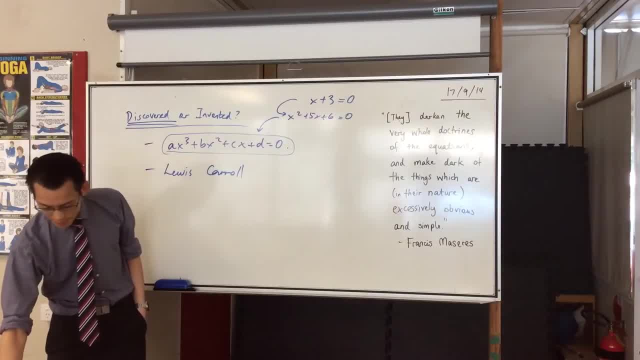 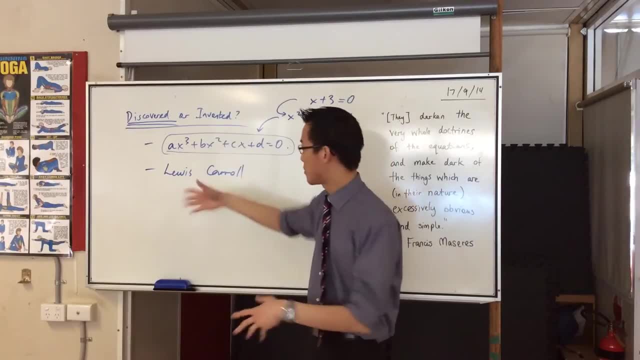 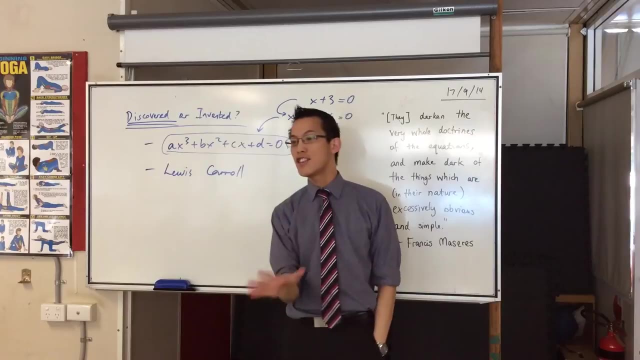 was. he said this sentence. I wonder what you think of this. In stark contrast to this guy right Talking about Lewis Carroll and the maths that he did, this presenter said maths is purely invention. Purely invention And the way he justified it. 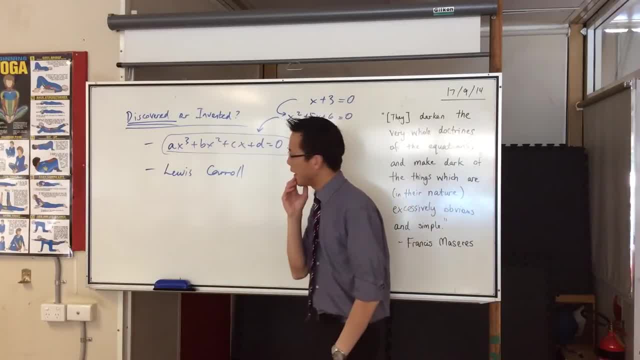 was this I was saying to you. maybe you want to write it down and have a think about it later. He said: think about the number three. I don't know why everyone picks three. Three's an important number, I guess. 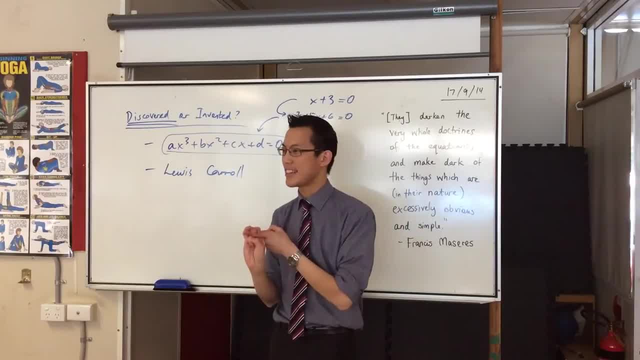 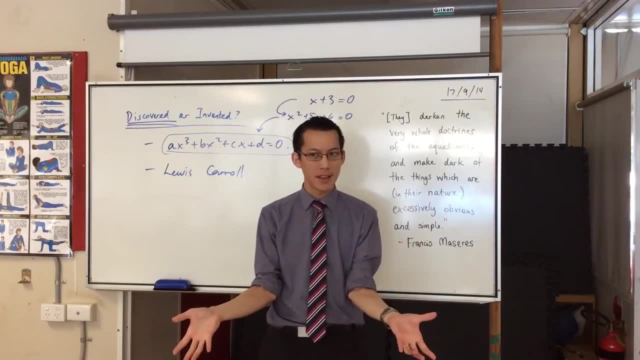 Think about the number three. Where does the number three exist? Where is the number three? Where can you point to and say: look, there's, that's three, that's what three is. Now see this. that's interesting, right. 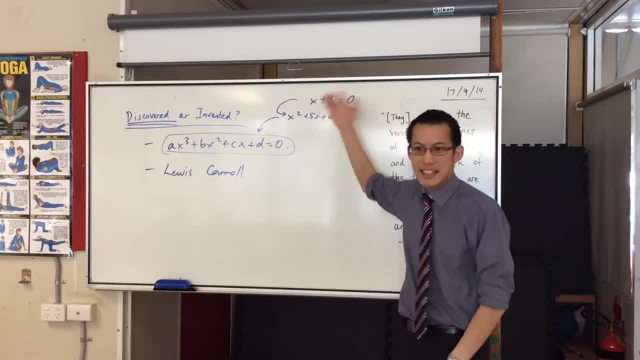 So that's a symbol that came out of my brain, right, Like it's not a it doesn't. it's there because I wrote it there, right? Where is it in reality? And the answer is: well, it exists. 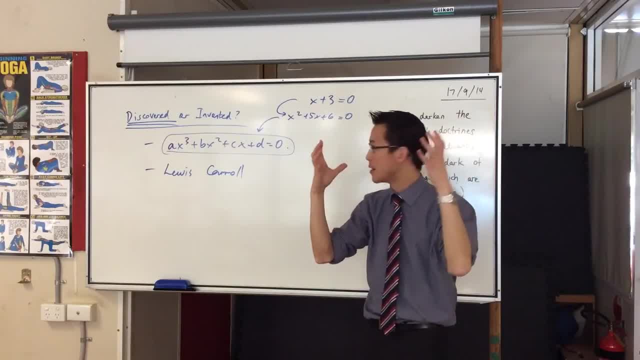 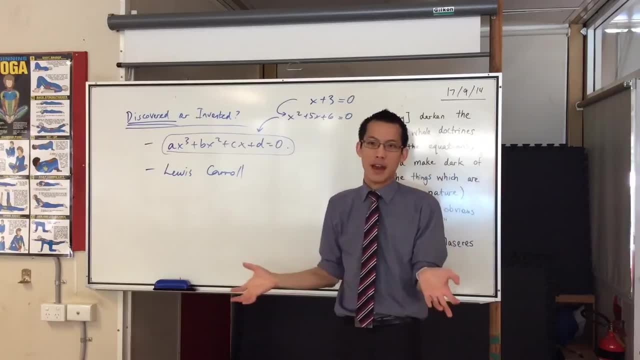 in human minds, right, Like that's where it comes from. It's an idea that we use and it's a symbol and all that kind of thing, but apart from that, it has no reality. You take humans away, you take three away, right, So that was. 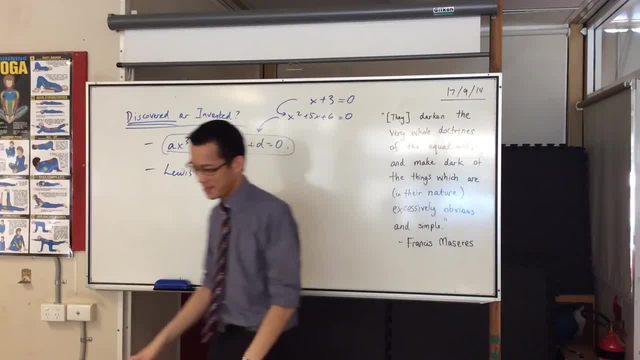 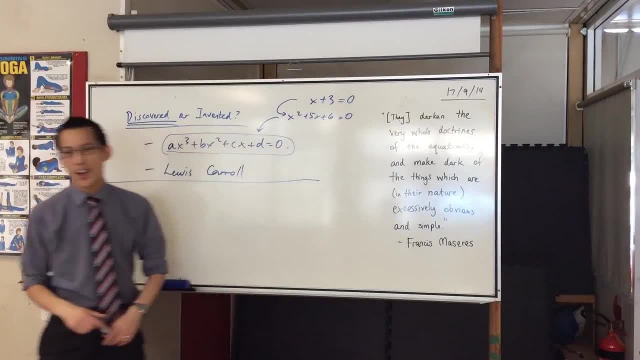 his argument for why it was completely invented. I thought that was super interesting. okay, So you can rule that off. Now here's this quote, which refers to something that we're going to cover today, which is on your handouts, Don't quite.